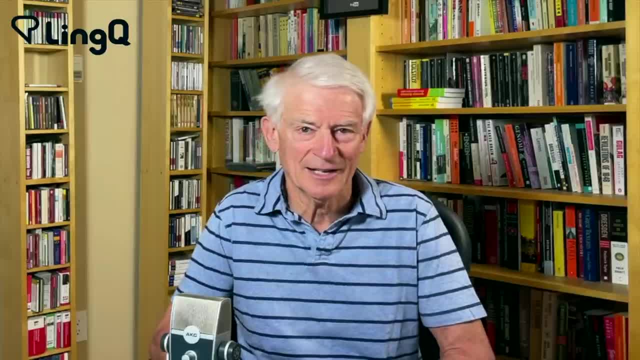 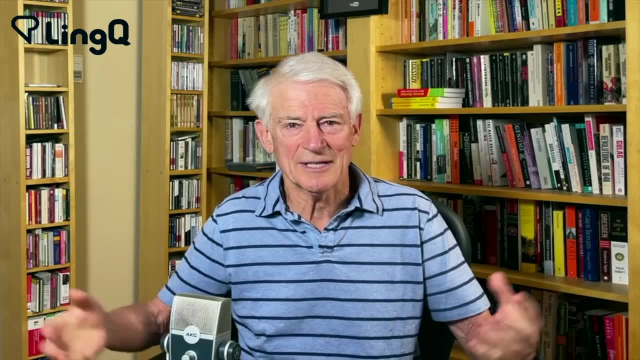 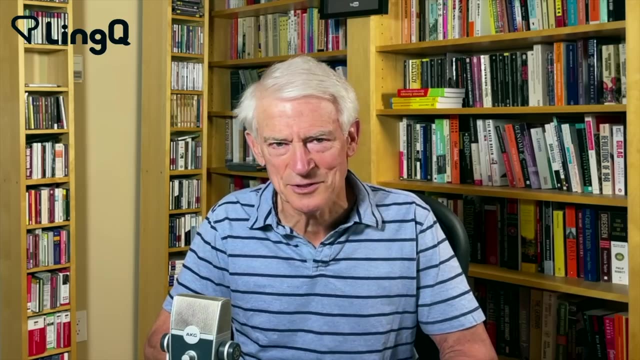 I always forget. And I study this sentence and I keep on forgetting And I thought to myself: yeah, you're not supposed to try to totally understand and remember that sentence, You're supposed to just allow the language to kind of enter your brain and let the brain get used to it. 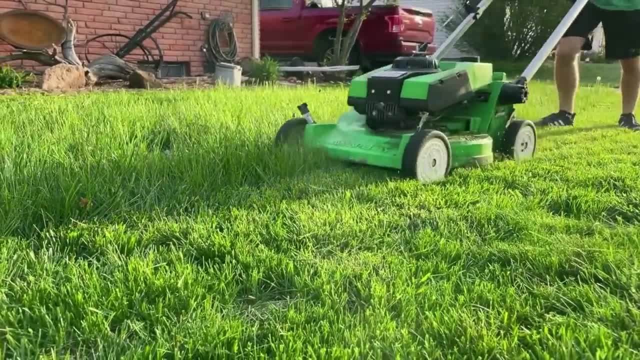 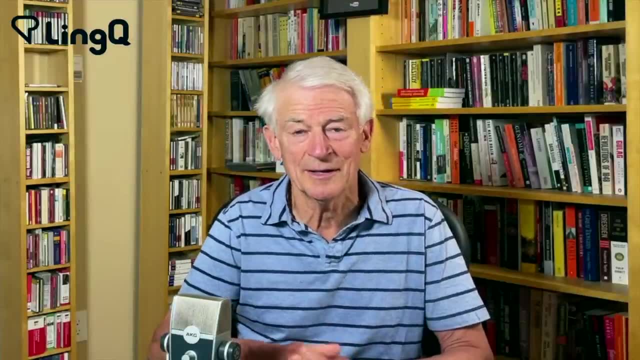 And so my brother said it's a bit like mowing a lawn. If the grass is high, then you have to set the lawn mower at a higher level in order to have an easier first pass. through mowing the lawn through, you can set the blades a little lower. 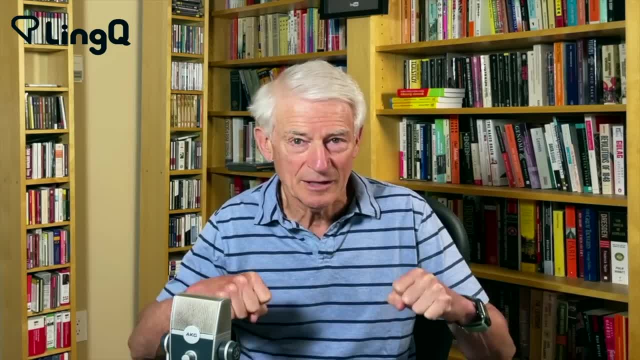 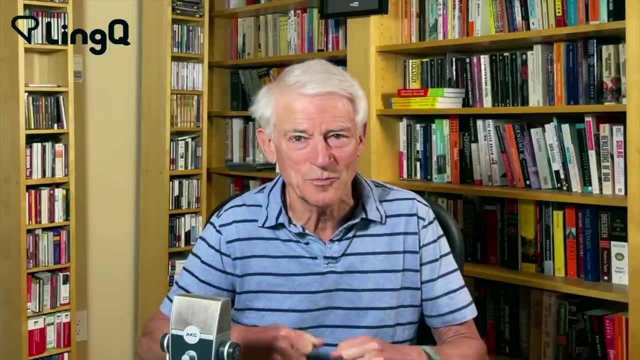 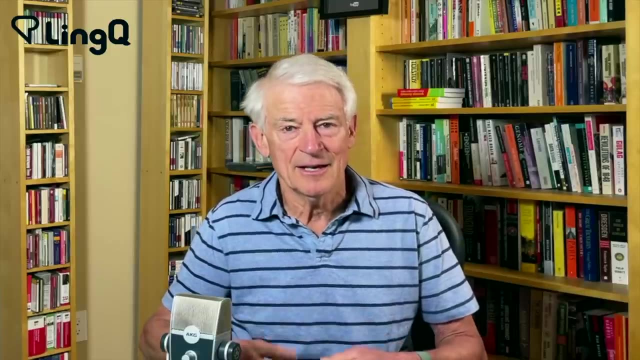 If you try to force yourself to push that lawnmower into very high grass, uh, you're not going to get there. It's going to be very hard work and you won't. you won't be able to to get the job done, depending on how long the grass is now in theory. if you have to mow the 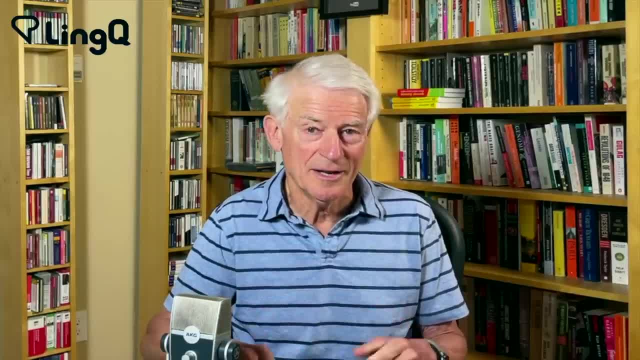 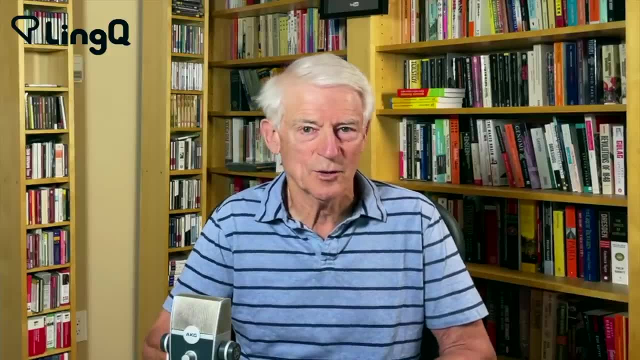 lawn twice, you would think it's going to take you twice as long. but if, in fact, there's just too much resistance and you can't mow the lawn, you're not going to get the job done. so it's far easier. 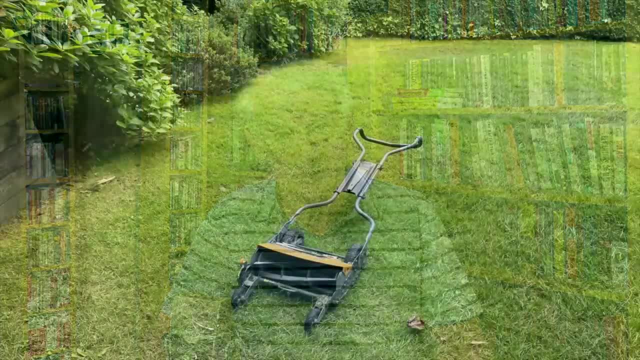 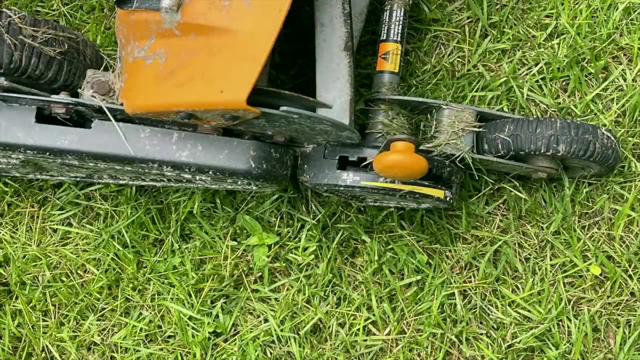 And I've had this experience and I'll show you the picture of my lawn and my lawnmower and how I adjust it, And it's much easier for me. particularly, we've had a lot of rain. I haven't been able to mow the lawn. 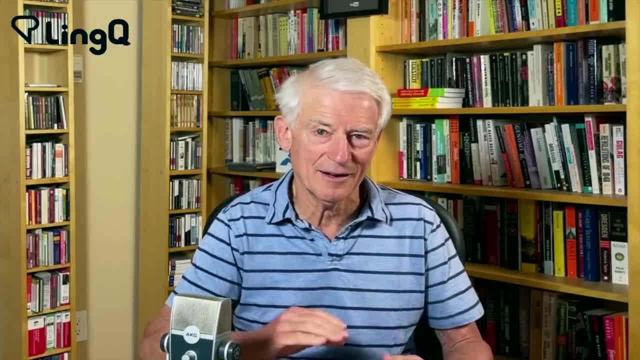 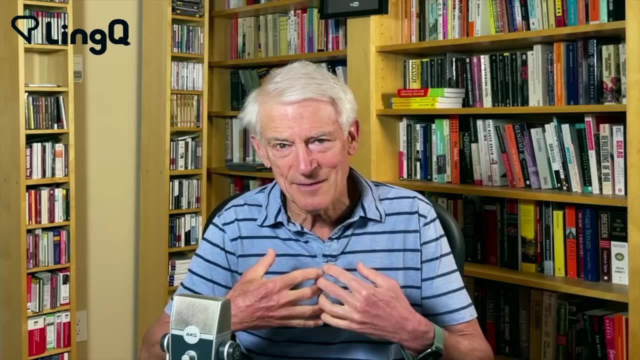 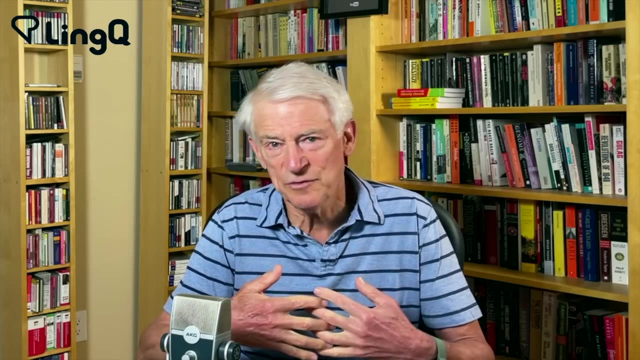 And so when I go in there I have a first pass at a higher level and then I have a second pass at a lower level. Every pass I pick up a little bit more. It's the same with the Content that I learned from listen to read. first time I go through I don't. 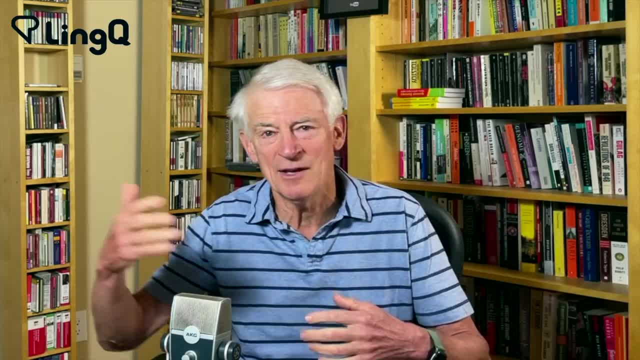 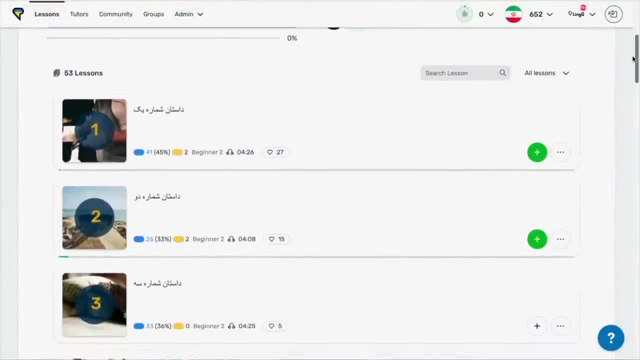 fully understand that I may listen a second time, I may move on to other lessons, And then I come back and even on something as basic as the mini stories, I always pick up something the second, third, fourth time through. so every time I mow that. 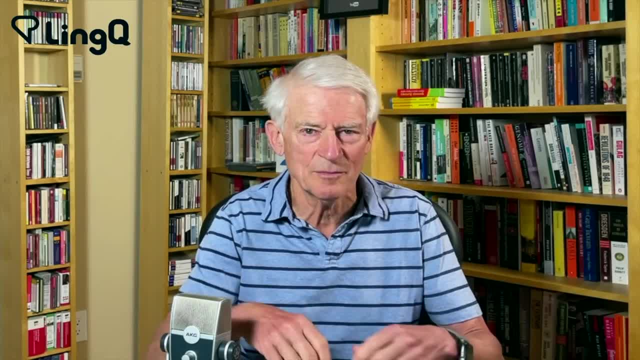 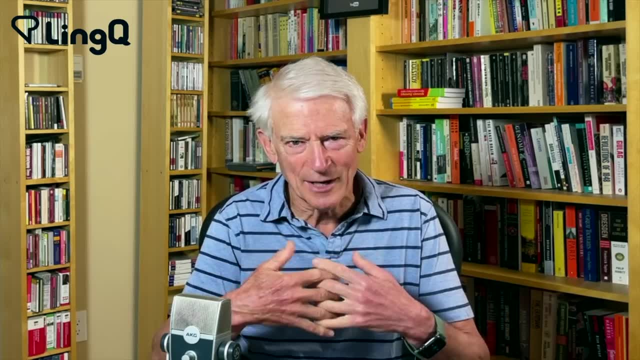 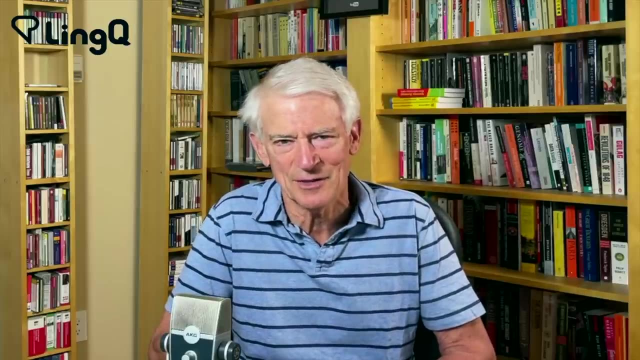 lawn. even I'm flowing through it. I'm pushing the mower through it easily, but I'm getting a few more blades Of grass and on. in that way, we will gradually enable our brains to get used to the language. Don't force yourself to try to understand. if you can't understand, move on to new material.